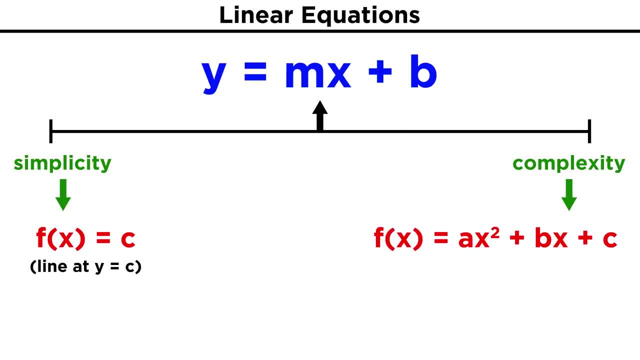 plus c. As we remember from algebra, solving these can be a little bit tricky. and if we look at cubic or quartic functions, or functions of higher degree still, things get quite a bit trickier. Linear equations are right in the middle, not too simple, not too complicated. which? 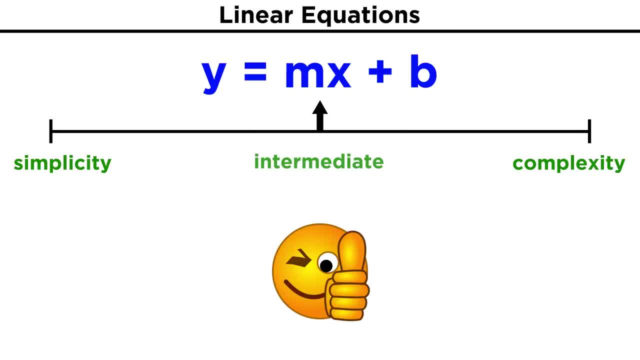 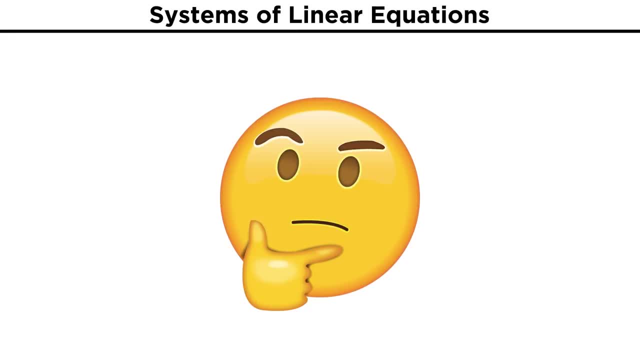 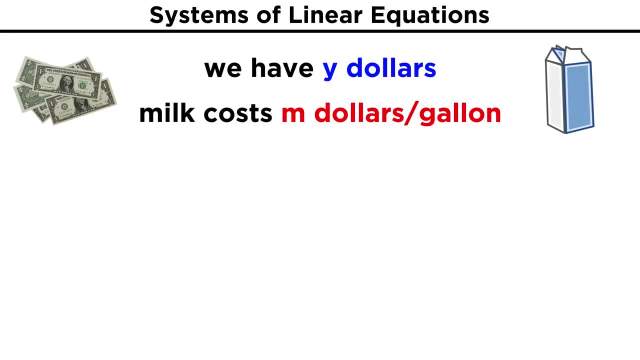 actually end up modeling a lot of real-world relationships To see how much structure we can get from linear equations. consider the following example: Say we need to buy some milk and we have y dollars. Milk costs m dollars per gallon, so how many gallons of milk can we get? 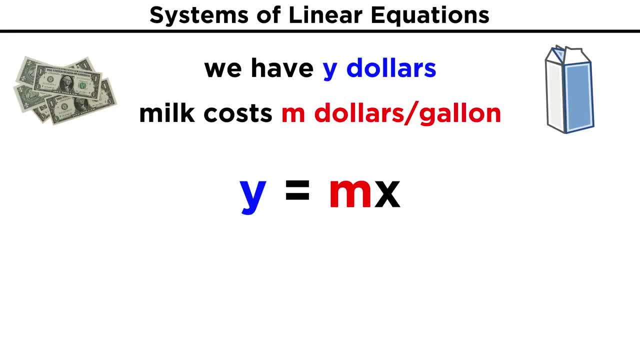 That's easy. we just set up the equation: y equals mx M dollars per gallon. times the x gallons we can afford will equal y the money we have. That's easy. we just set up the equation: y equals mx M dollars per gallon. times the x gallons we can afford will equal y the money we have. 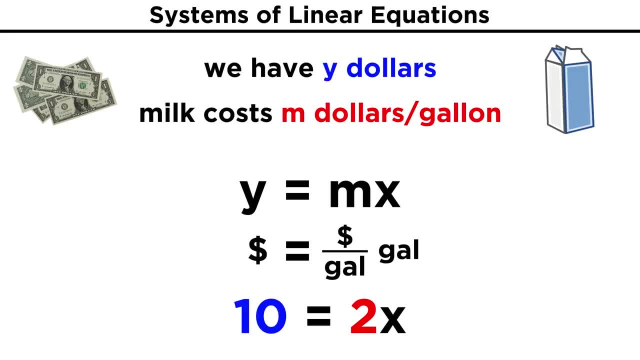 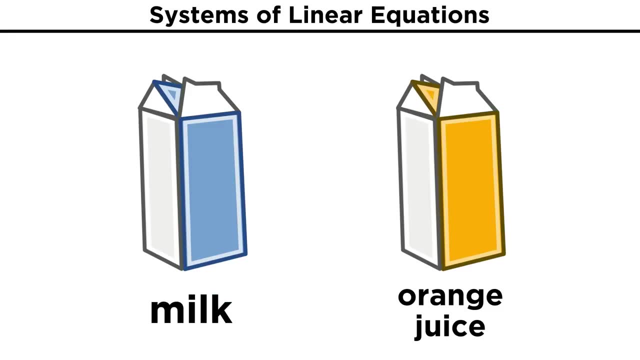 If m is two dollars per gallon and y is ten dollars, since we have ten dollars, ten divided by two is five and x equals five. We can get five gallons of milk with our ten dollars. Now let's step things up a little. 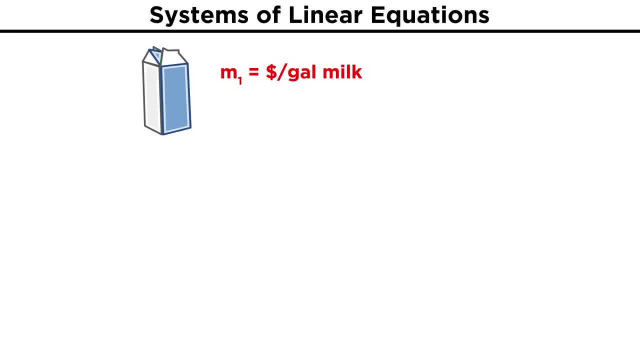 Perhaps we also need to get some orange juice. Let's say that m1 is the cost of milk per gallon and x1 is the number of gallons of milk we get. M2 is the cost of milk, M2 is the cost of orange juice per gallon and x2 is the number of gallons of orange. 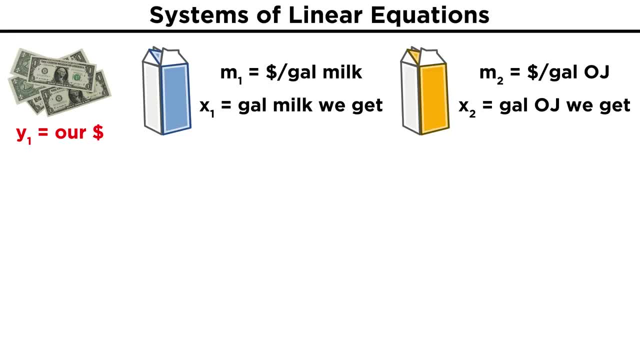 juice we get. Y1 is the amount of money we have, and so y1 will equal m1x1 plus m2x2.. All of a sudden, there are infinitely many options for what to do, as there are infinite combinations of x1 and x2 that will satisfy this equation. 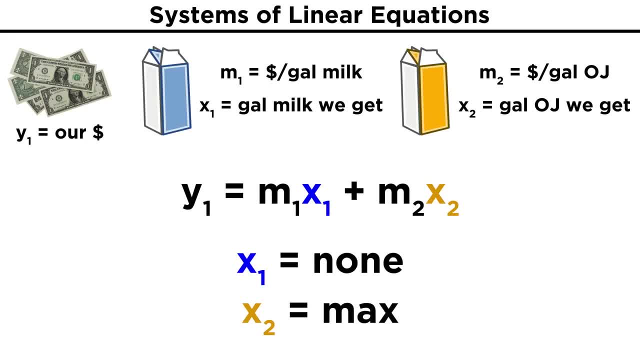 We could buy no orange juice and lots of milk, Or we could buy no milk and lots of milk, Or we could buy no orange juice, Or, more likely, we could buy some combination of milk and orange juice. but we can choose any value for one of these and then calculate the other. 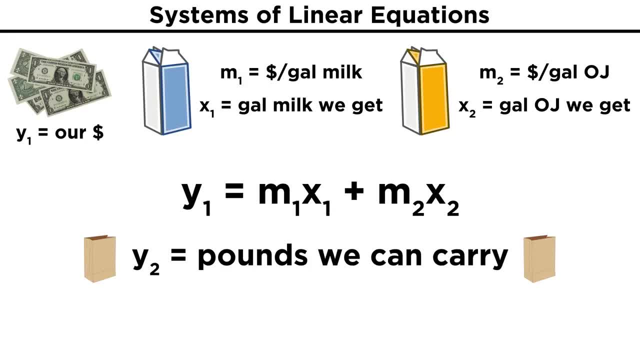 Now let's throw another parameter in there. Let's say we can only carry y2 pounds of stuff home with us. Milk weighs w1 pounds per gallon and orange juice weighs w2 pounds per gallon. That means that y2 equals w1x1 plus m2x2.. 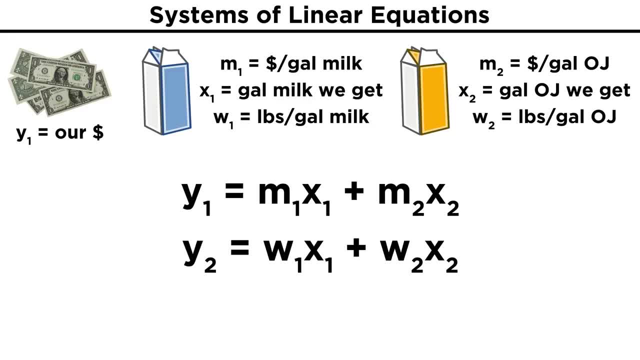 That means that y2 equals w1x1 plus m2x2.. That means that y2 equals w1x1 plus m2x2.. Now we need values for x1 and x2 that satisfy both equations simultaneously. So things are starting to get a little more complicated, but let's note that each of 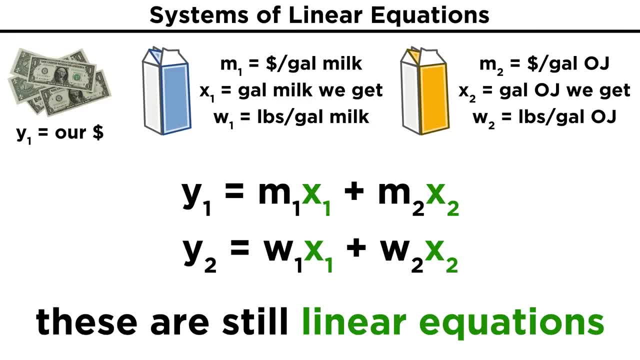 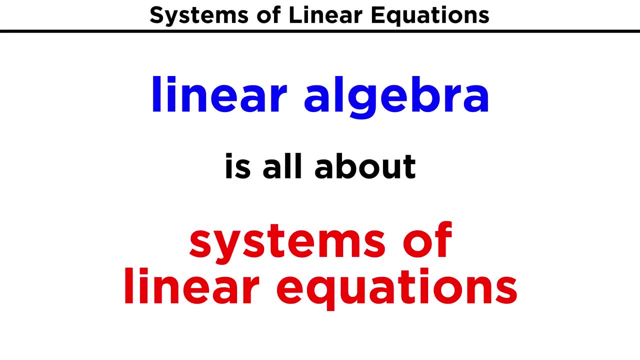 these is still a linear equation. This means that everywhere we see x, it is not being raised to any exponent, but since there is more than one equation, we can call this a system of linear equations. As you can probably guess, we will be looking at all kinds of different systems of linear 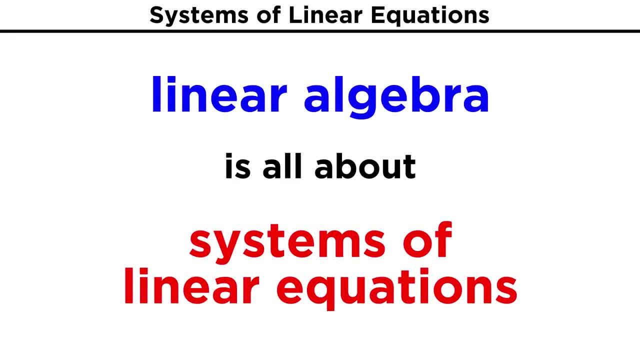 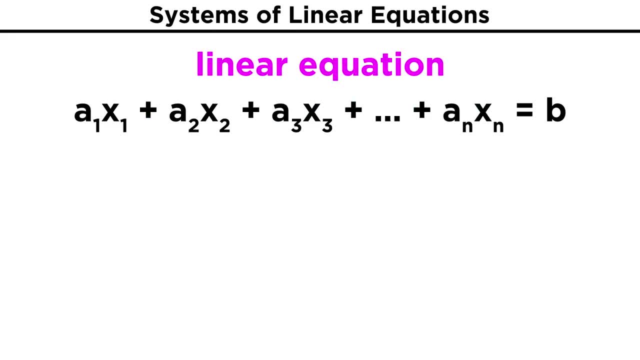 equations as we study linear algebra. For this reason, let's get some basic definitions and terminology out of the way regarding linear equations. From now on, we will consider a linear equation to be any equation in the form a1x1 plus a2x2. 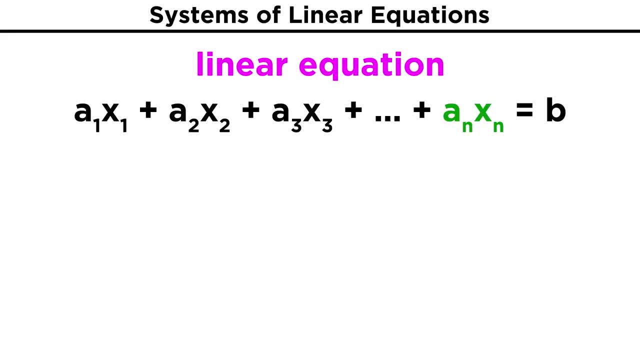 plus a3x3, all the way to anxn, equals b. So, as we can see from the ellipses, there can be any number of terms of this type, depending on the value of n, and their sum will equal some constant. 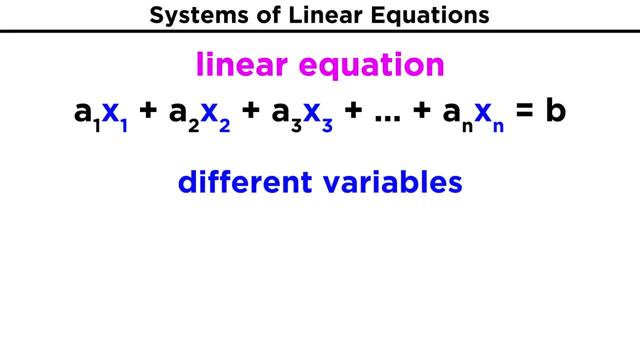 The A terms are coefficients of any type and the X terms are not all X. they are actually all different variables. They could be A, B, C and so forth, or more commonly, X, Y and Z, if there are just three. 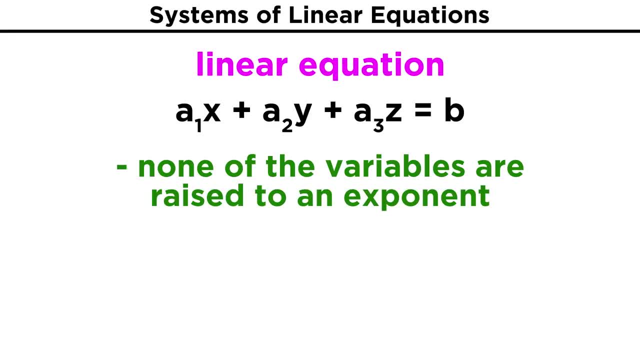 The main thing that must be true is that none of the variables are raised to any exponent. otherwise it would no longer be a linear equation. it would be a quadratic or cubic or something else. Also, there are no roots, no trigonometric functions, none of the other more complicated. 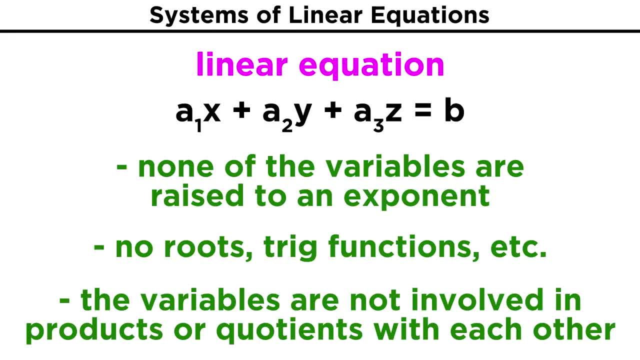 functions we have learned are going to be involved here. In addition, none of the variables are involved in products or quotients with each other. there is just a series of individual terms that are not related to each other. So in that sense, systems of linear equations are very simple. 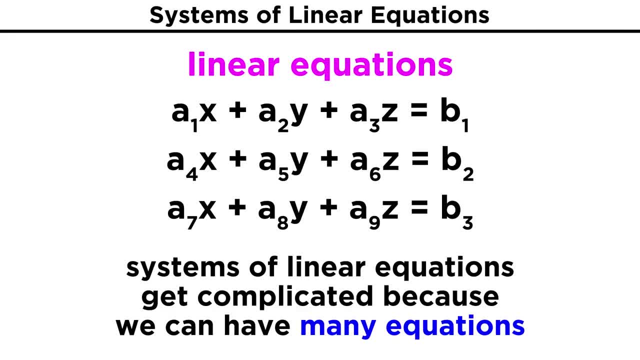 They get complex in other ways, namely due to the fact that if we have three equations involving three variables, as is shown here, we will have to use certain techniques to solve this system. A solution to a system of linear equations will have as many values in it as there are. 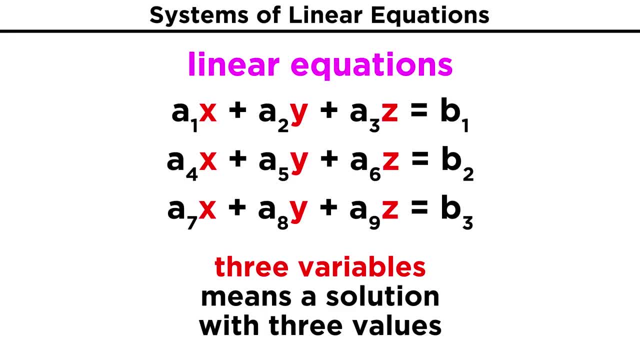 variables in the system. In other words, we need a value for each variable. In other words, we need a value for each variable. In other words, we need a value for each variable that will make all of the equations true at the same time. 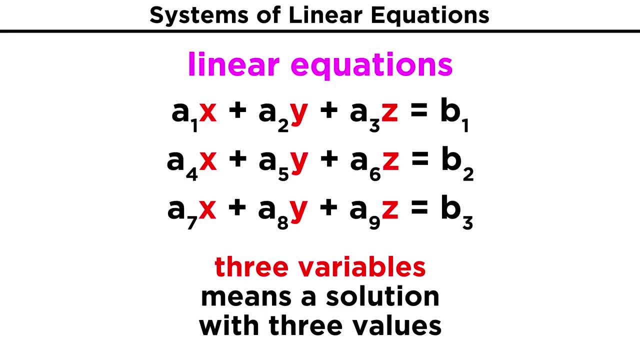 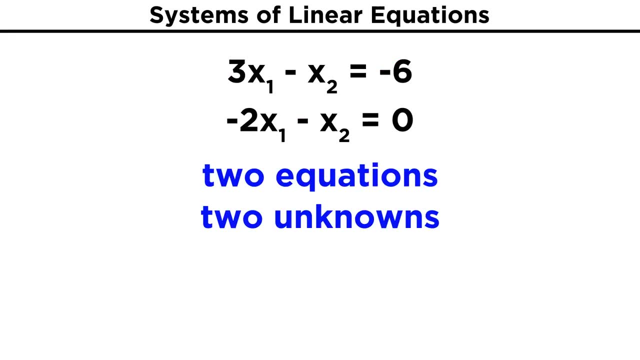 And there is no limit to the number of variables or equations in a system. so that is the sense in which systems of linear equations can get very complicated, despite the fact that each individual equation is extremely simple. But at first we will look at very simple systems, some that are as simple as two equations. 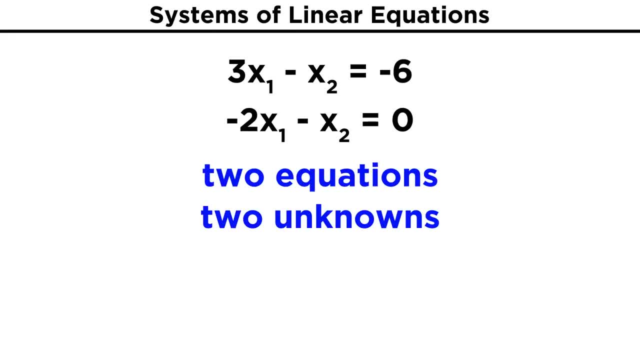 with two unknowns which we learned how to solve when we studied algebra. Take something like three x one minus x two equals negative six and negative two x one minus x two equals zero. We can take x one and x two to be the same thing as x and y, so we can just solve these. 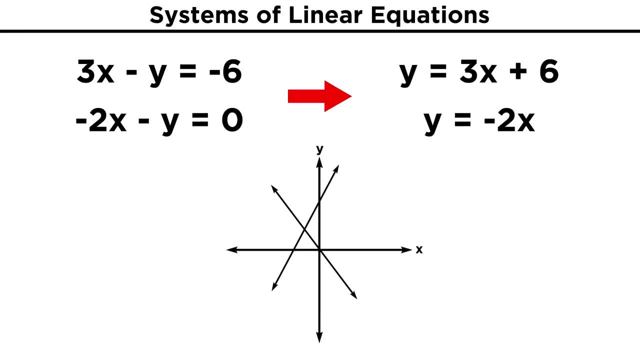 for y and graph the lines, We will get y equals three x plus six and y equals negative two x. If one line is all the points that satisfy one equation and the other line is all the points that satisfy the other equation, then we will get y equals three x plus six and y equals negative two x. 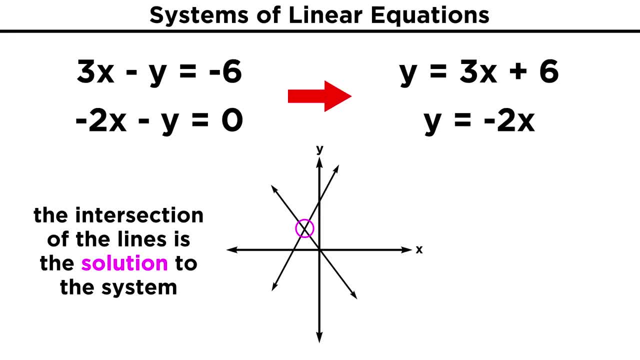 If one line is all the points that satisfy the other equation, then the point at which they intersect is the solution for the linear system, as the coordinates of that point give us the x one and x- two values that satisfy both equations in the system. 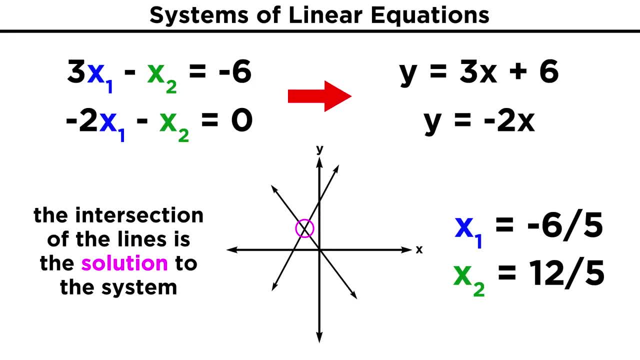 If we go through the algebra, we would arrive at negative- six fifths for x one and twelve fifths for x two, and that's the unique solution to the system. If we had two lines that were parallel, there would be zero solutions to the system, and 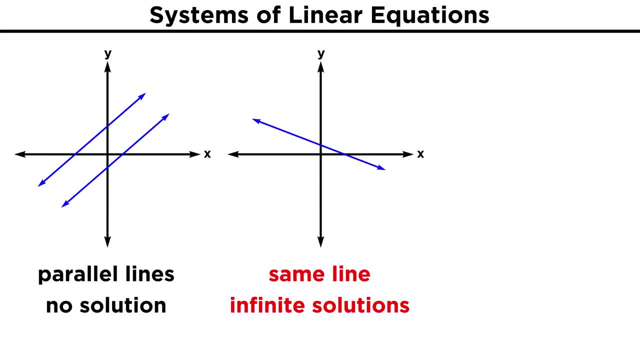 if two equations were different ways of expressing the same line, there would be infinitely many solutions to the system. as we recall from algebra, When a system has at least one solution, we say the system is consistent, and when a system has no solution, we say that the system is inconsistent.